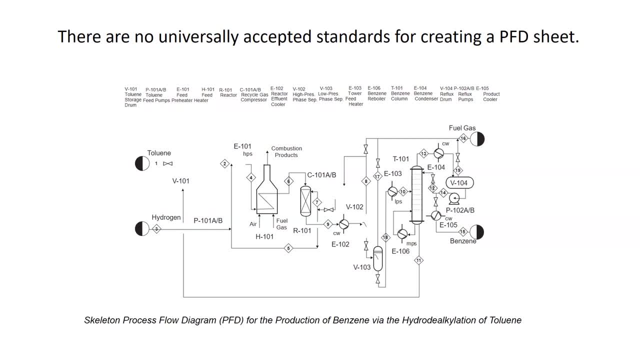 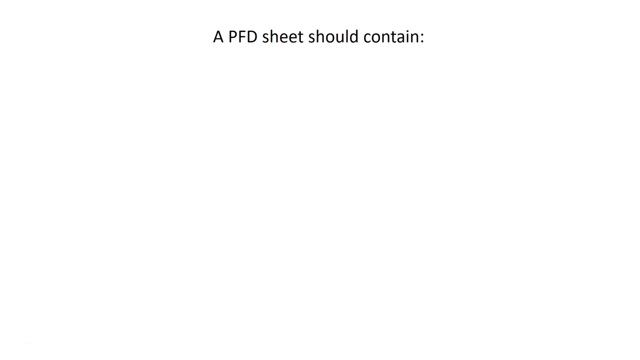 different information from the PFD for the same process from another company. Having made this point, it is fair to say that most PFDs convey very similar information. commercial PFD will contain the following information: All the major pieces of equipment in the process will be presented on the diagram along with. 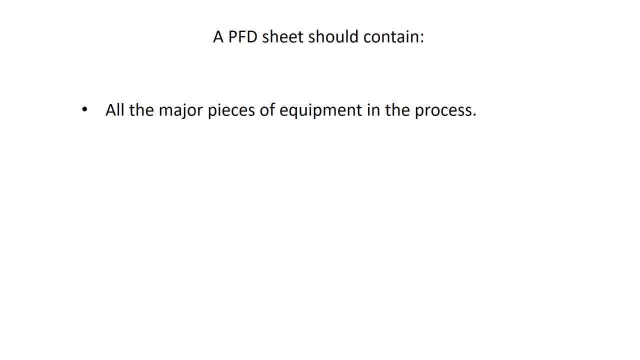 the description of the equipment. Each piece of equipment will have a unique equipment number and a descriptive name. Secondly, all process flow streams will be shown and identified by a number. The description of the process condition and chemical composition of each stream will be included. These data will be either: 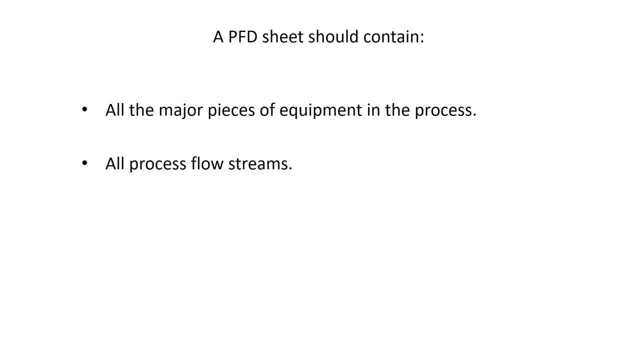 displayed directly on the PFD or using a stream table. Finally, all utility streams supplied to major equipment that provide a process function must be shown as well. It is clear that the PFD is a more complex diagram than PFD. a BFD or block flow diagram require a substantial effort to prepare. 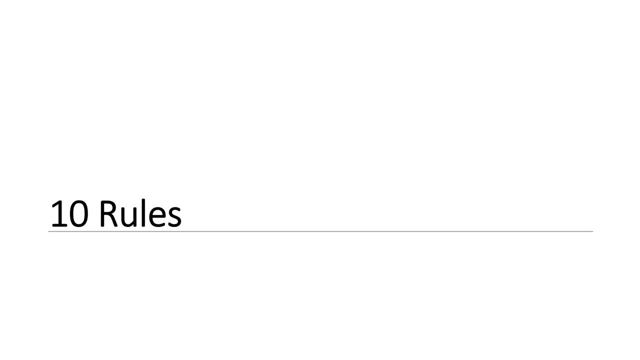 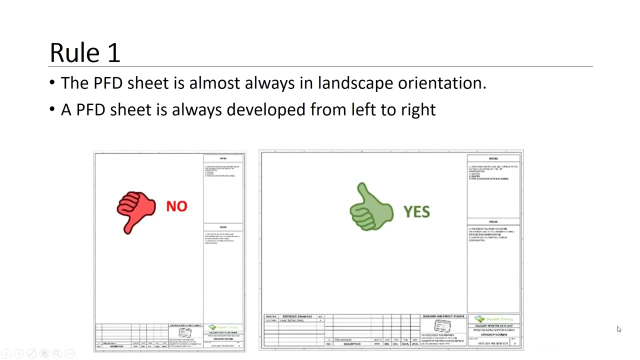 It is essential that it should remain uncluttered and be easy to follow to avoid errors in presentation and in interpretation. Now I'm going to describe 10 simple rules for you. If you follow these simple rules, it will help you to create good quality BFDs. Rule number one: Your BFD. 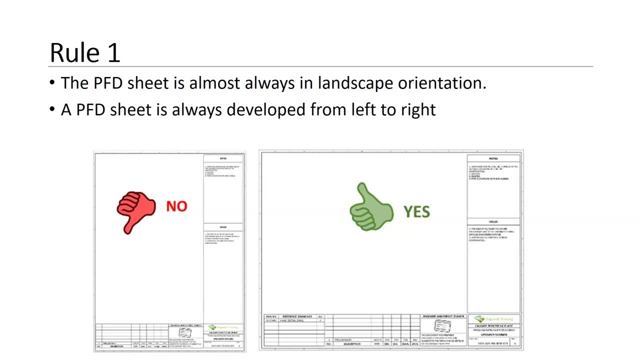 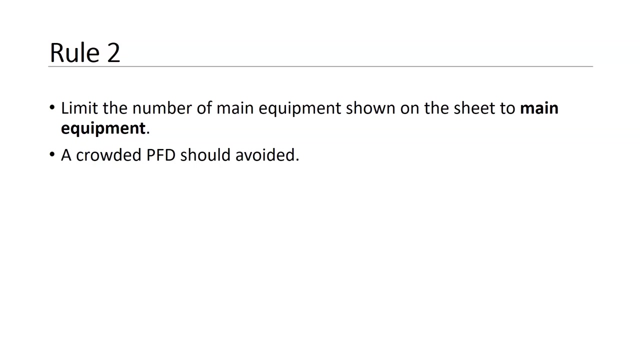 sheet should be in landscape orientation. You should develop it from left to right, top to bottom, So avoid any portrait orientation when you are developing your BFD sheet. Rule number two: Limit the number of main equipment you are showing on your sheet. 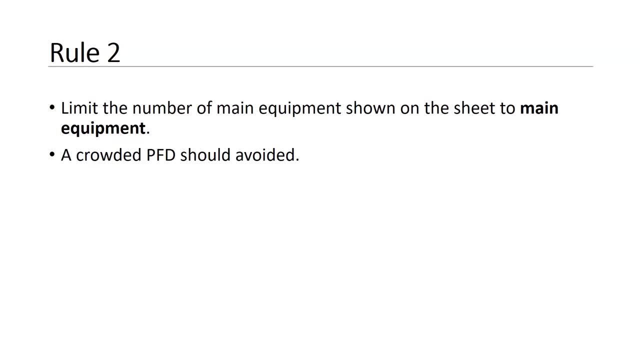 Stick to the main equipment. Avoid crowding or overcrowding your BFD. BFD should be simple and easy to understand. You should be able to follow the streams. Rule number three: Your BFD is a diagram of your process. It is a 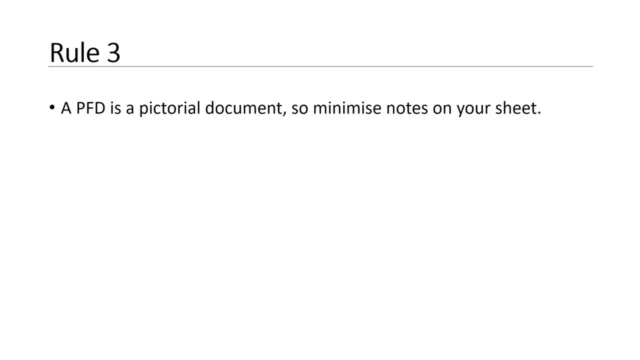 pictorial document. So minimize number of the notes or text that you put on your sheet. So you have to only put major equipment in the process on your sheet: all the process flow streams, all the utility streams and services and finally only essential valves, not all the valves or control instruments. 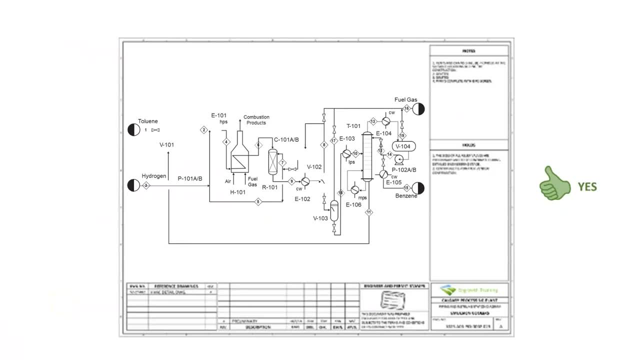 Let me show you another example. This is a very good example of a high quality BFD. You can see all the major equipment and the process streams are on the sheet, plus the major and essential valves. Also, as you can see, it is developed from left to right. 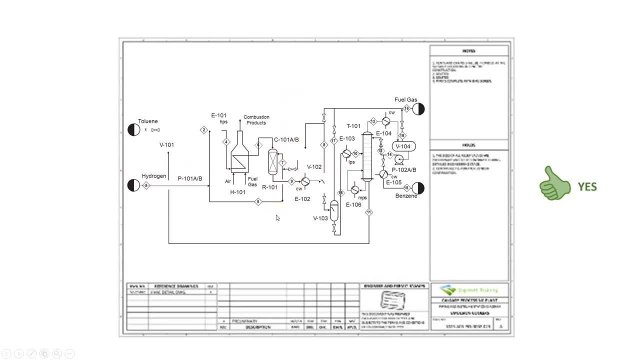 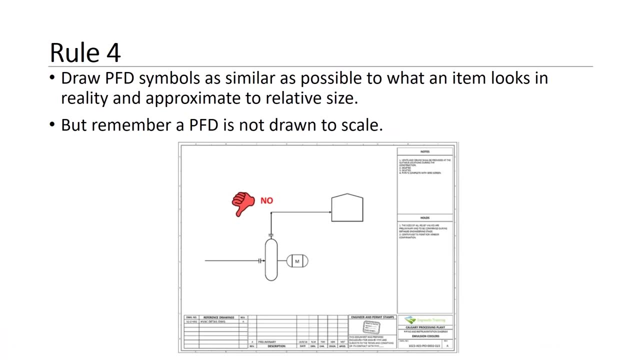 top to bottom and it is not to the scale. Remember pfd is not the scale. rule number four: draw pfd symbols as similar as possible to what an item looks in reality for columns, tanks, heat exchangers etc. and remember it is not to the scale. 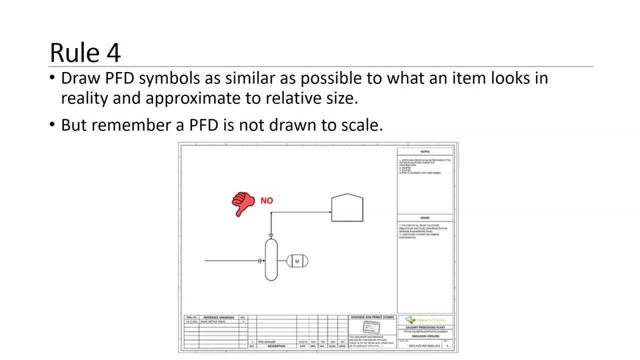 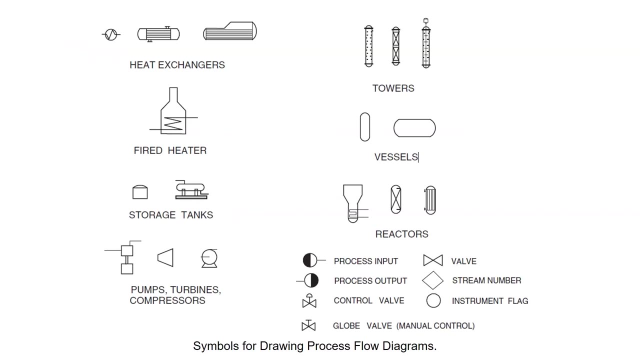 so it is a d size document. there is no standard for symbols. most of the companies possibly have got their own and standards. those symbols are available in the the tools that uh engineers are using and they draw them from the libraries and then add them to the m sheet. there are standard. 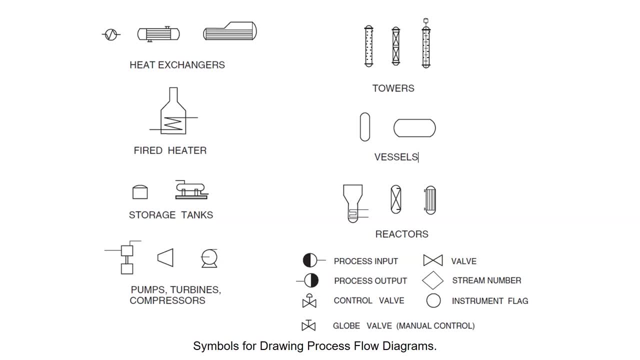 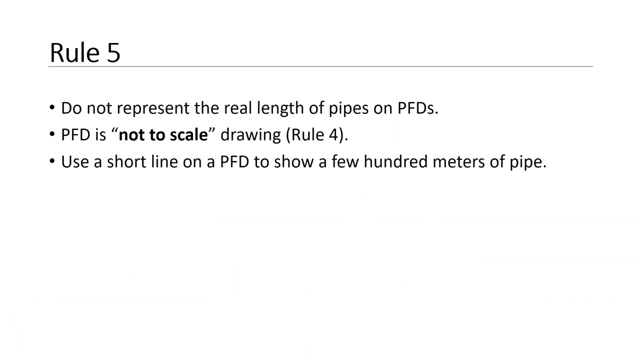 softwares like autocad or others that engineers are using these days, but also depends on what standards the companies are using. um it's have to follow the guidelines as well. rule number five, as mentioned, pfd is not to scale drawing. remember the previous rule. so if you have got 100 meters of the pipe, you don't need to represent that on your pfd. 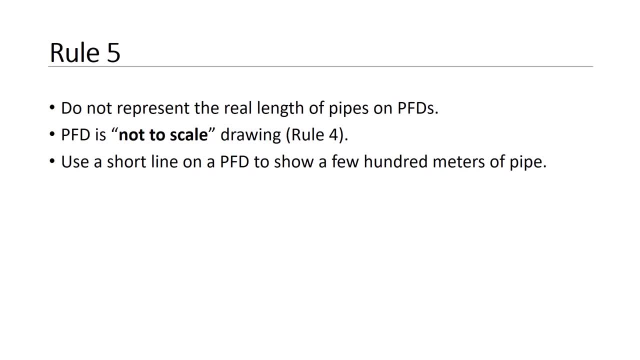 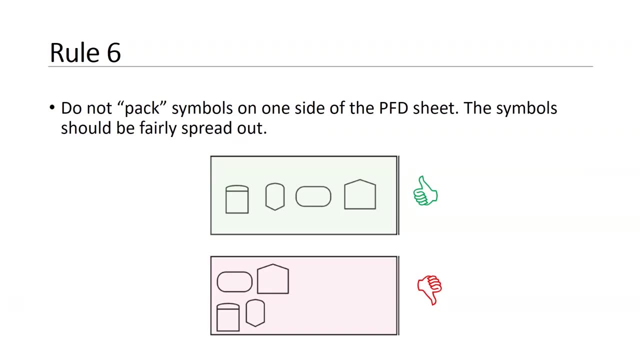 use a short line on a pfd to show a few hundred meters of the pipe. rule number six: do not pack symbols on one side of the pfd sheet. the symbol should be fairly spread out throughout your um working area. avoid cluttering and your pfd shape. it should be uncluttered. 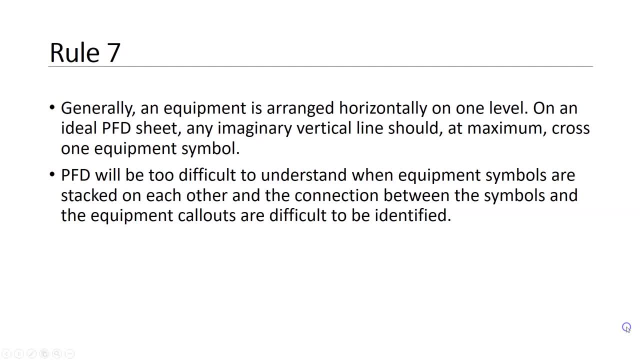 and clear and easy to follow. rule number seven: generally an equipment is arranged horizontally on one level. always develop your sheet left to right, top to bottom. on an ideal pfd sheet, any vertical line should at maximum plus one equipment symbol. pfd will be too difficult to understand. 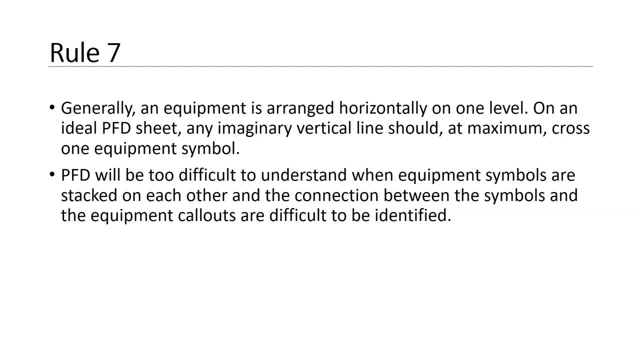 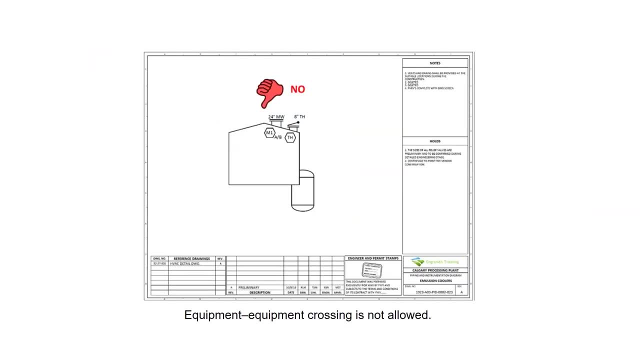 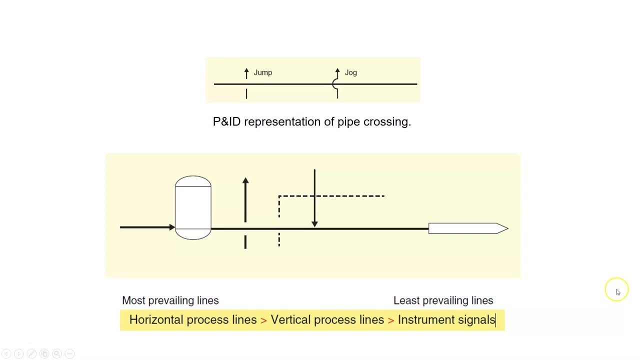 when equipment symbols are stacked on each other and the connection between the symbols and the equipment call outs are difficult to be identified. this is a very good example that the two equipment on on top of each other avoided in your pfd sheet. when the streams or lines are crossing, there are two different ways that you can represent them on your 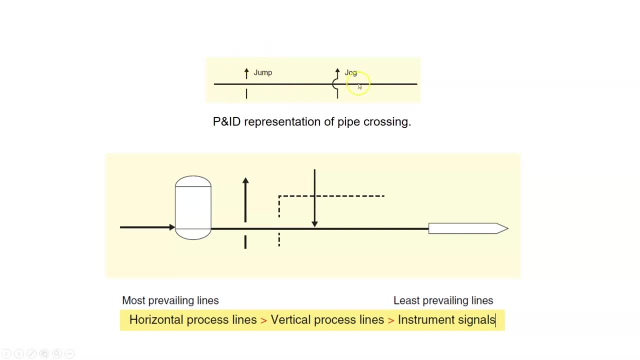 pfd sheet. you can use a jump method or a jogging one, doesn't matter which one you use, but stick to one method. be consistent on your pfd sheet. also, remember, in terms of the priority: the highest priority are with their horizontal process lines and then vertical process line. 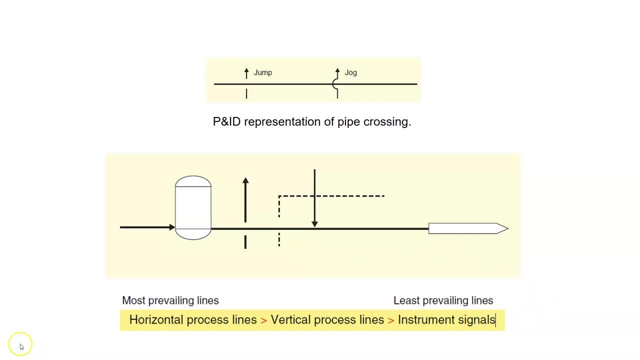 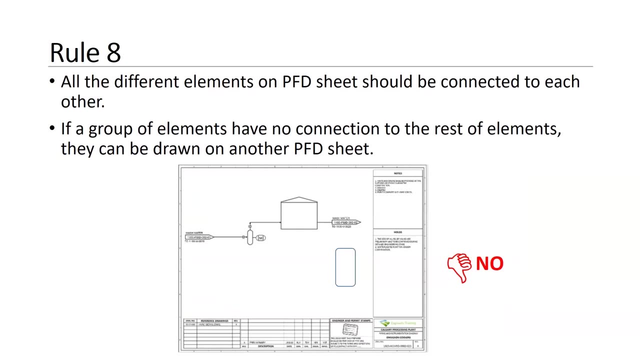 and then vertical process line and vertical process line and vertical process line and vertical process line. rule number eight: all the different elements on pfd sheet should be connected to each other. so if you have got a one equipment or a group of element with no connection to the rest of 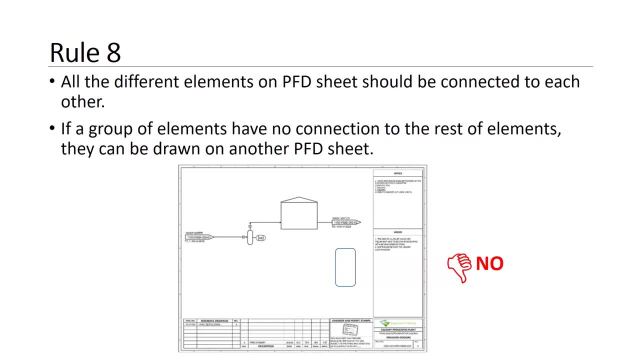 the process, then avoid putting them on your pfd sheet. maybe they should be on the different pfd sheet but not on that one. this good example that you can see. there is a one equipment, for example. it's the column which is not connected to the rest of the process. it shouldn't be there. 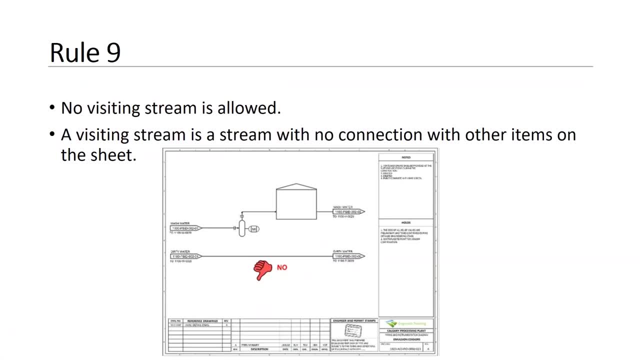 simply following rule number eight, make sure there is no visiting a stream on your pfd sheet. a visiting stream is a stream with no connection with other items on the sheet. for example, on this example you see that there is a a visiting stream which it comes and leaves the the diagram without a.